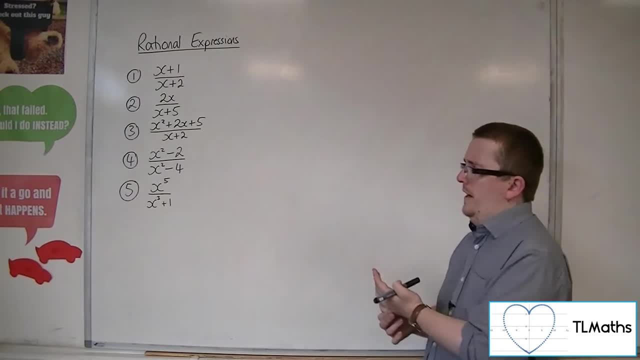 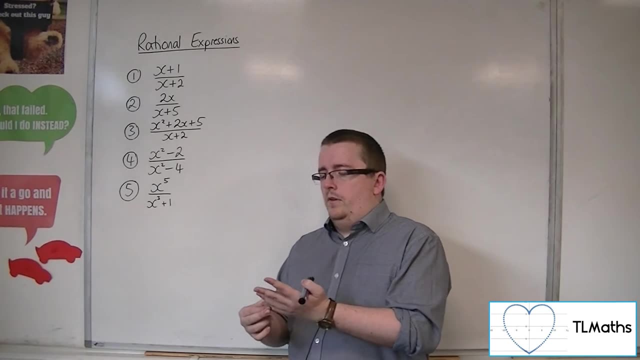 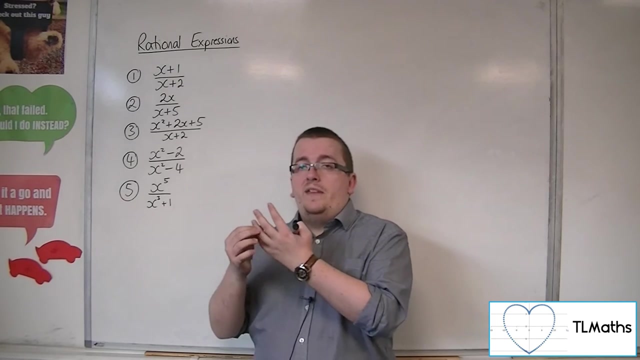 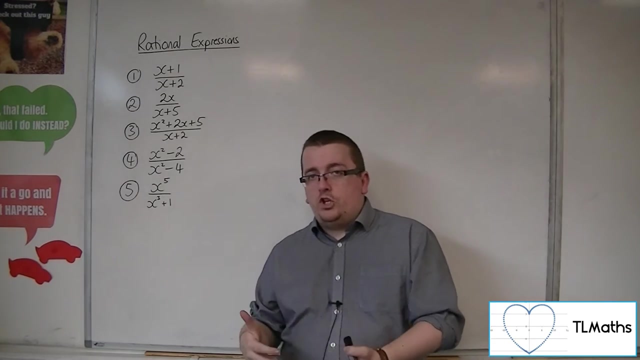 Or in a simpler form. Some of these will still be a severe problem, of course, for integration, But this process can certainly help. The other is understanding about the analysis of the function and thinking about what the function looks like, especially what it behaves like as x increases over time. 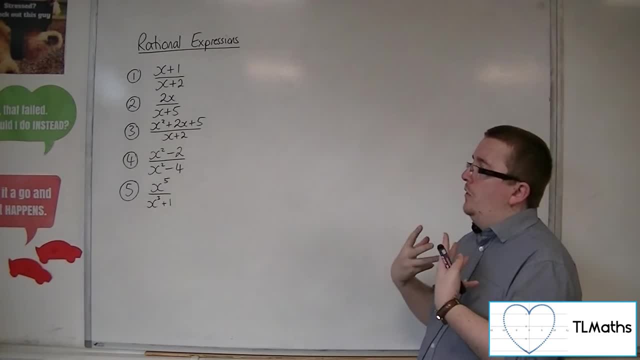 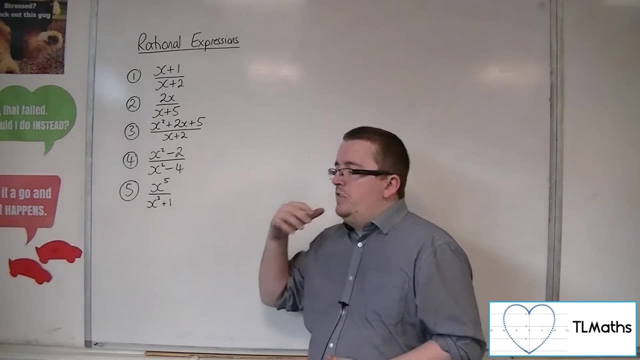 So this is really the methodology. if you really wanted to go into how to sketch graphs and move forward with that, Then knowing how to do polynomial division for these rational functions, you can then look at: well, the curve will approach another curve. 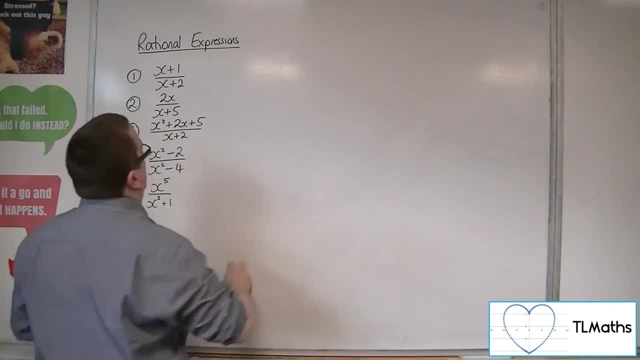 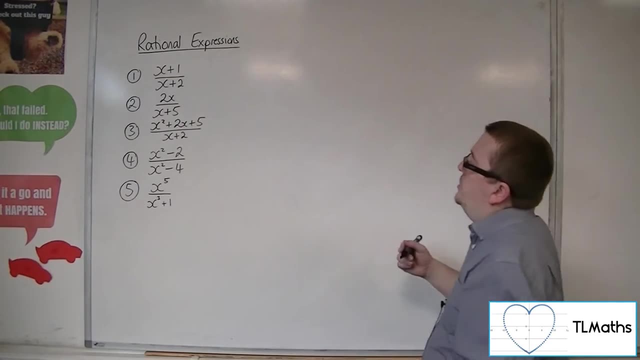 So we'll see some examples of that as we work through this. So, for example, if I had x plus 1 over x plus 2. Then I can still use polynomial division. I can write x plus 2 down the left-hand side. 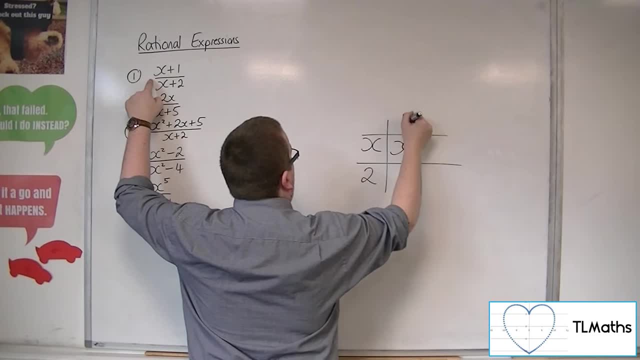 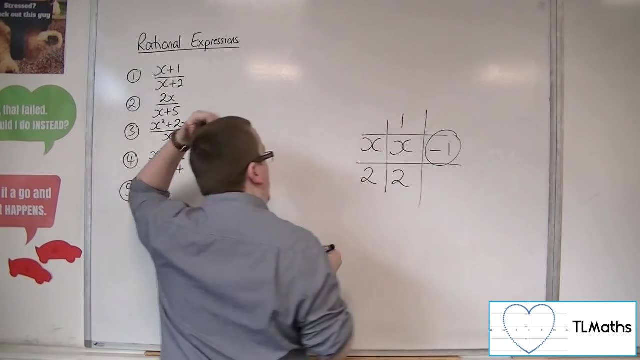 And I need to have x, so x would go there, So that would be 1.. 1 out of 2 is 2. And I need 1, so I'm going to have to subtract 1 away. So that's my remainder. 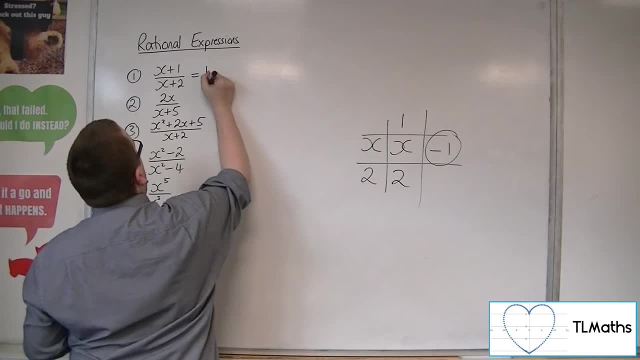 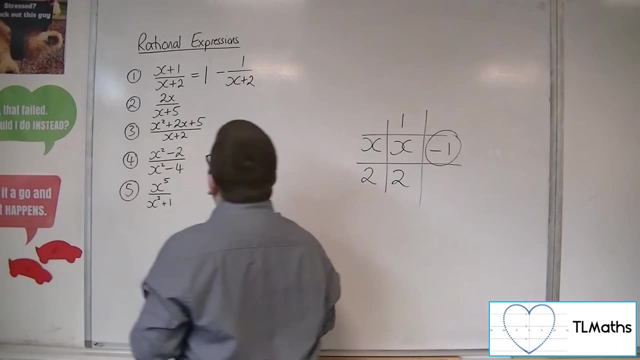 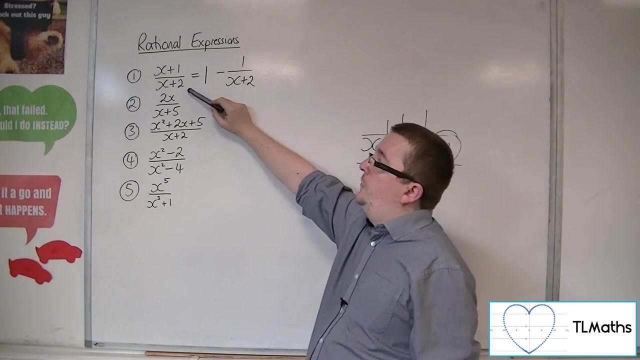 So I get 1.. And the remainder is minus 1. So take away 1 over the x plus 2.. So what this is telling me is that this function here, if I had a y, equals x plus 1 over x plus 2, and I decided to sketch it. 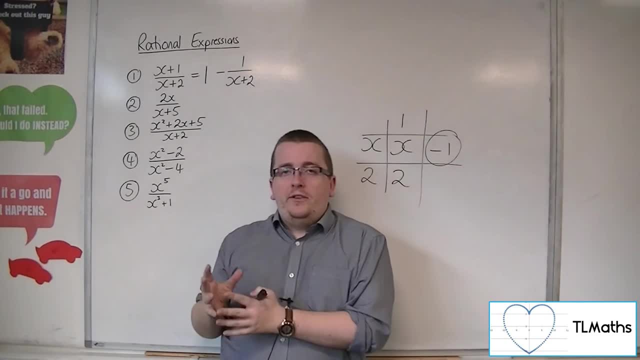 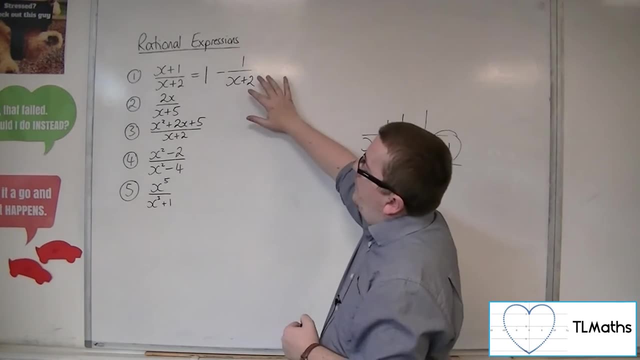 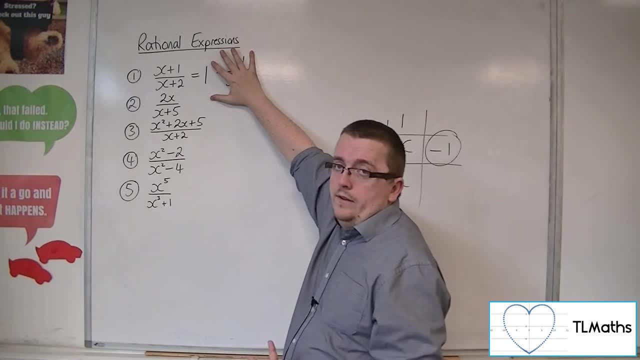 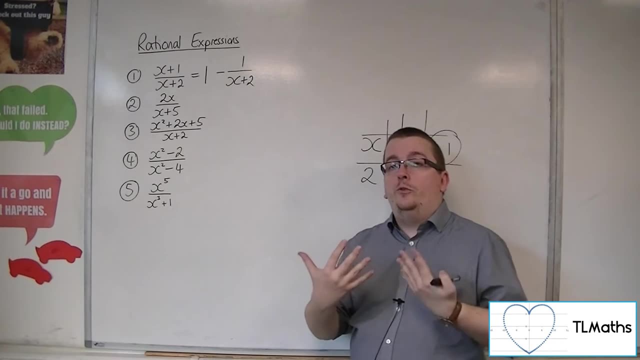 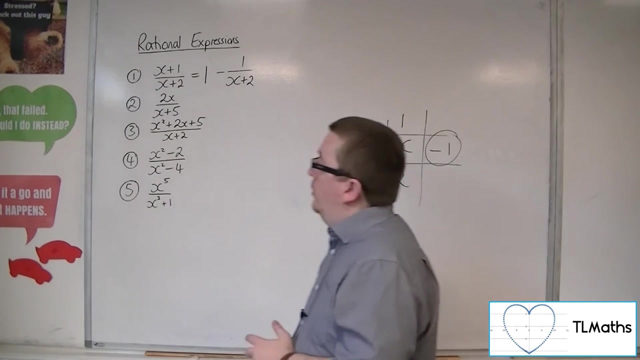 this function gets closer and closer and closer to 1.. So just the line y equals 1.. And so I know that y equals 1 is actually a horizontal asymptote that the curve is approaching. So I can use this polynomial division to show that. 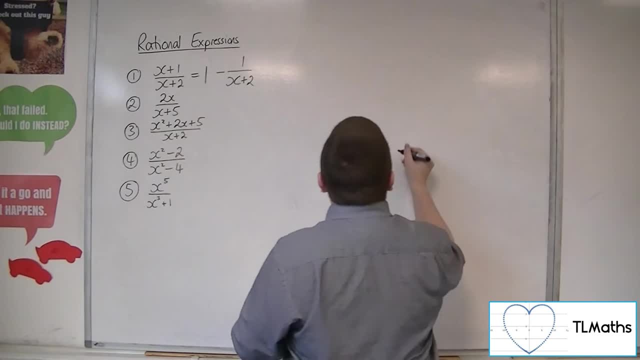 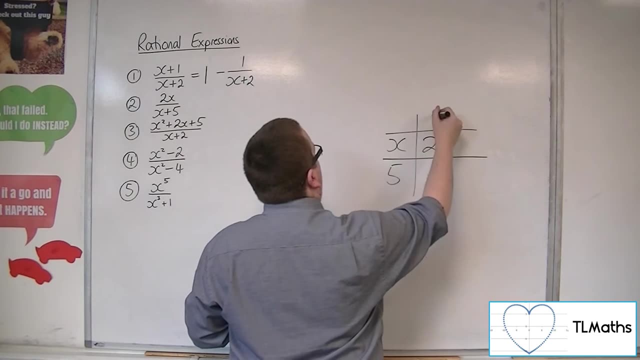 So if I now do 2x over x plus 5, I have x plus 5 down the left-hand side. I want the 2x, So x's into that go 2.. 2- lots of 5 are 10.. 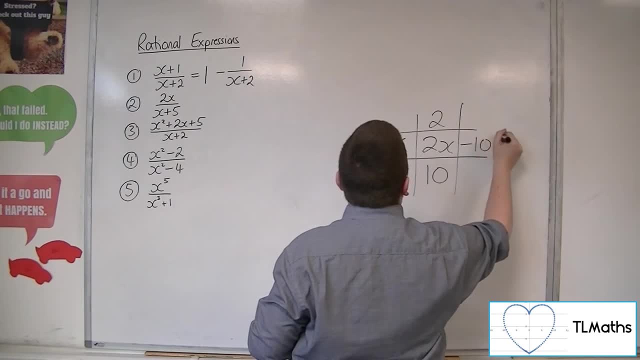 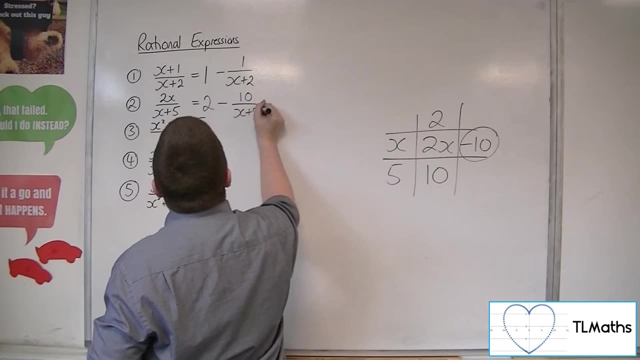 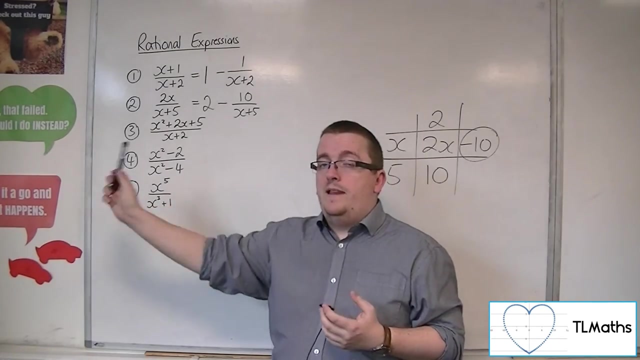 I don't have anything there, so I'm going to have to subtract 10.. So this would be 2 take away 10 over x plus 5.. So for this curve as x increases, or even if it's going into the left, 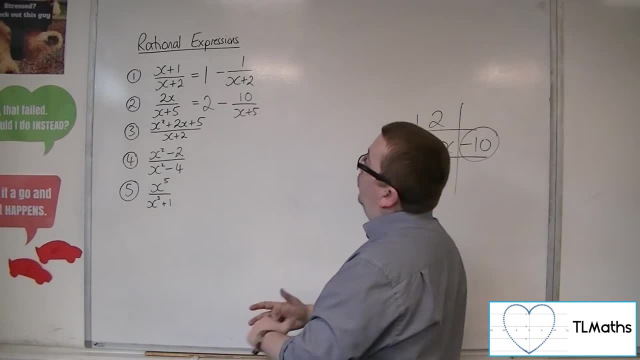 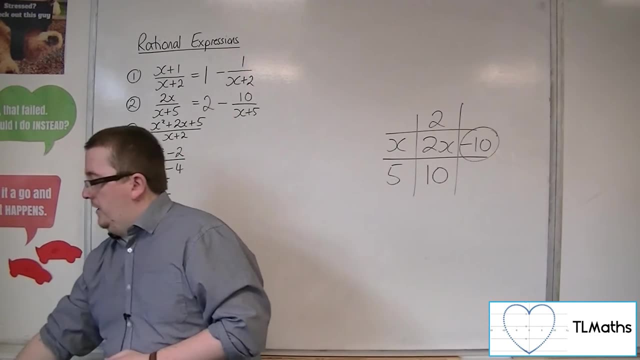 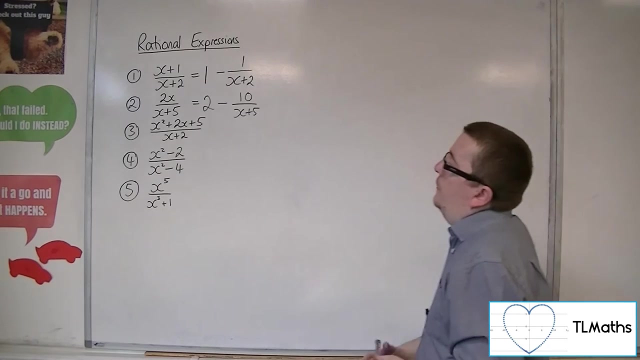 so as x is increasing, but in the negative direction as well, this curve will tend. this curve will tend to change towards y equals 2.. Okay, And so I can see that as a horizontal asymptote. Now for x squared plus 2x plus 5, over x plus 2,. 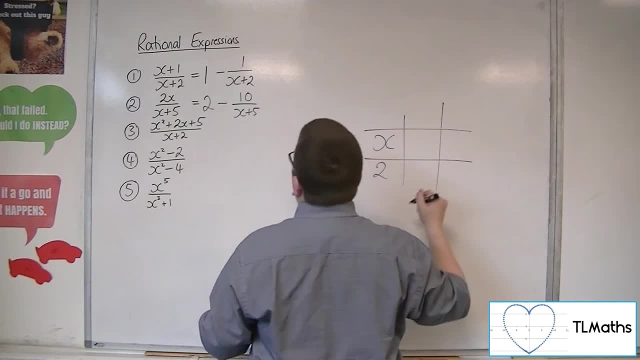 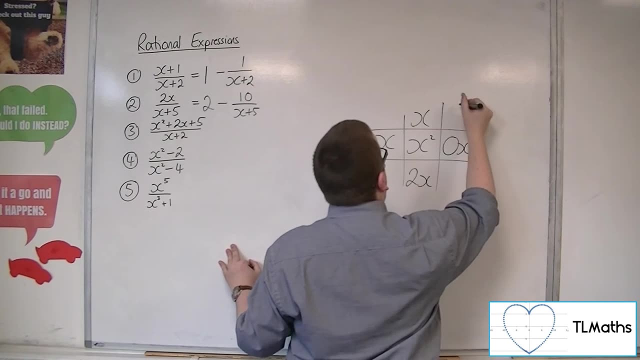 x plus 2 on the left-hand side will have x squared, So x there, 2x there. I've already got a 2x, so that'll be 0x, So that'll be 0.. That'll be 0.. 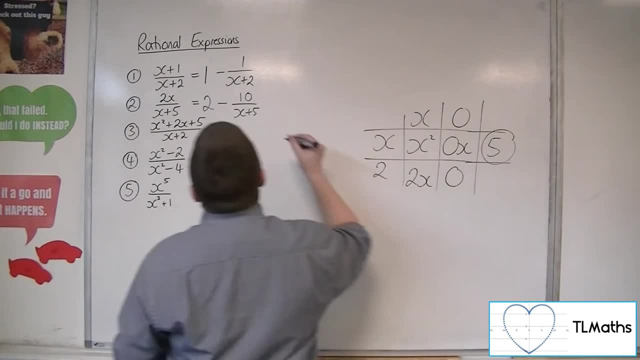 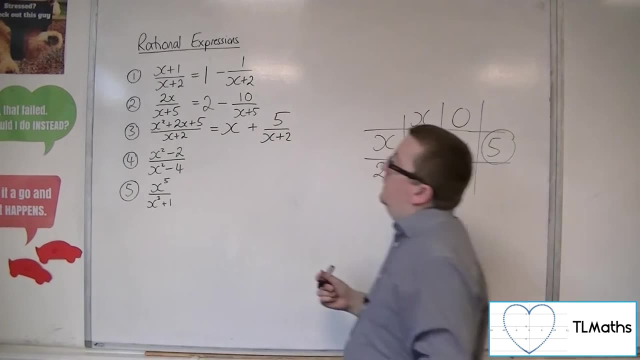 I don't want 0 there, I want 5.. So I'm going to have a 5 remainder. So this is equal to x plus 5 over x plus 2.. The remainder was 5.. So what that means is that for this curve, 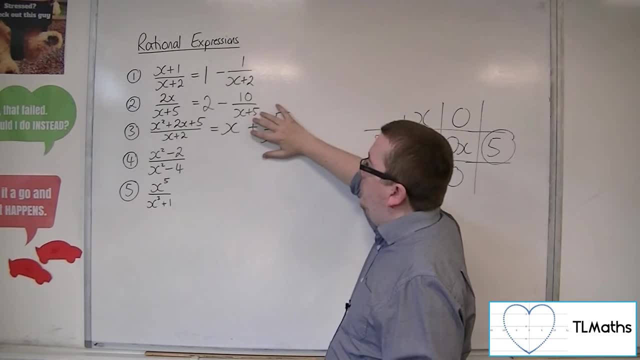 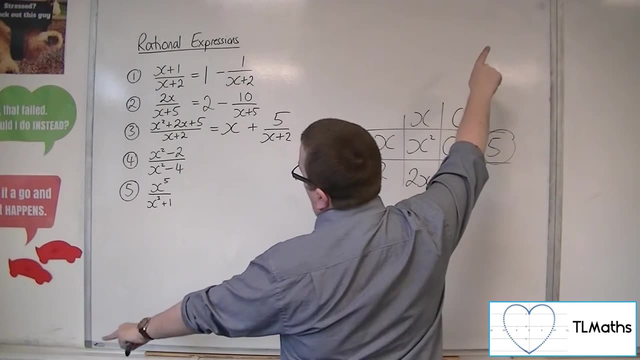 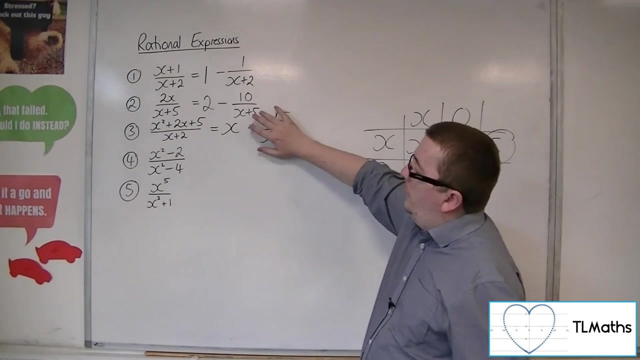 as x increases, it starts to behave like y equals x. So it approaches the diagonal line: y equals x as x tends to infinity. Okay, In either direction. So it's quite interesting. So close to minus 2, obviously something horrible is happening. 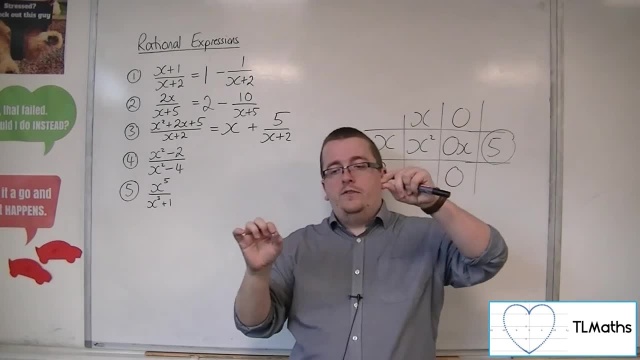 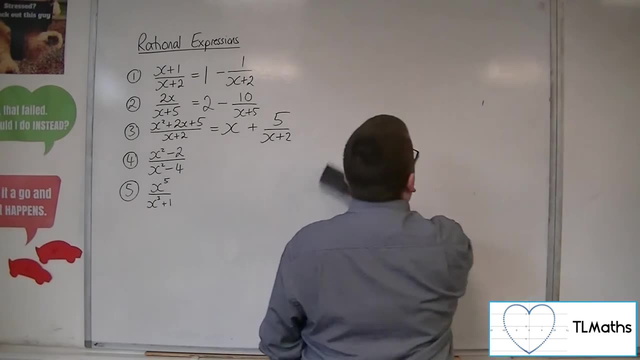 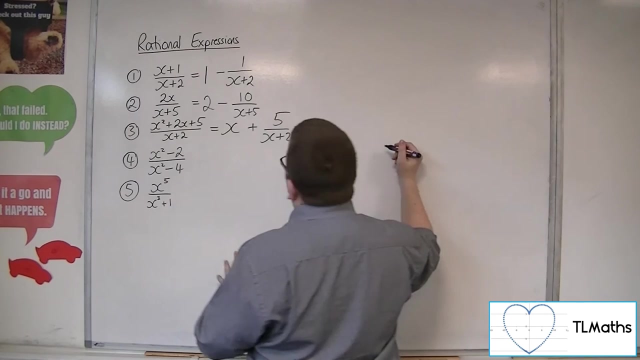 But as you get further and further and further away, this curve will start to look like the diagonal line: y equals x, And this is what this analysis can tell you. So number 4, x squared minus 2 over x squared minus 4.. 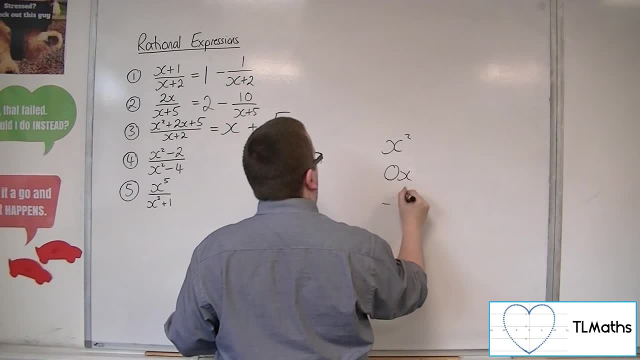 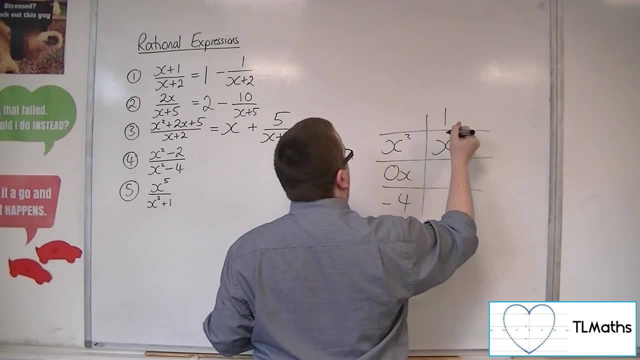 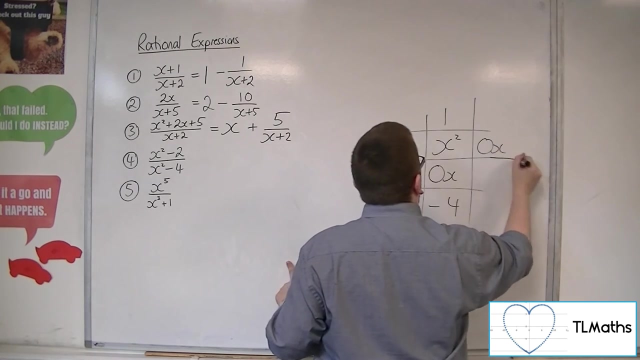 So x squared, 0x of minus 4. down the left-hand side, x squared, so that'd have to be 1. So 0x and minus 4.. So I don't want any x's, That's fine. 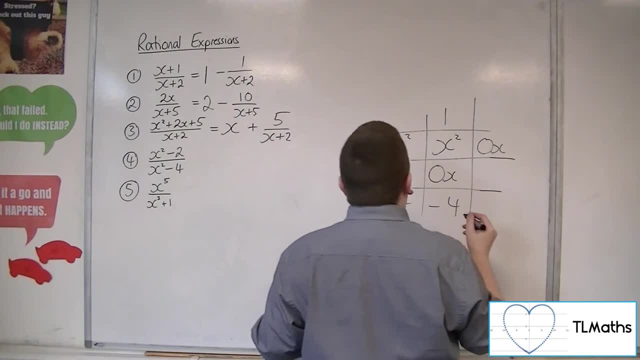 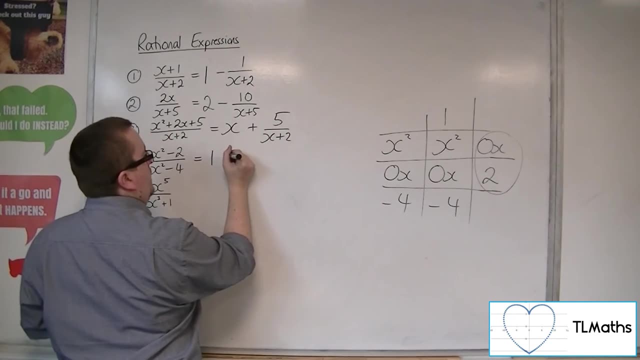 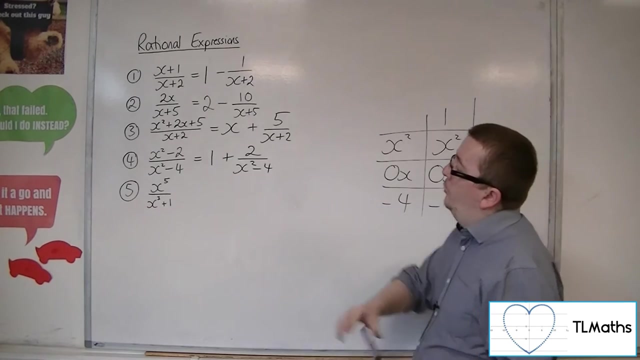 But I want minus 2.. So I'm going to have to have a positive 2 there. So I've got this remainder. So this would be 1 plus 2 over x squared minus 4.. So this curve clearly tends towards y equals 1 as x increases. 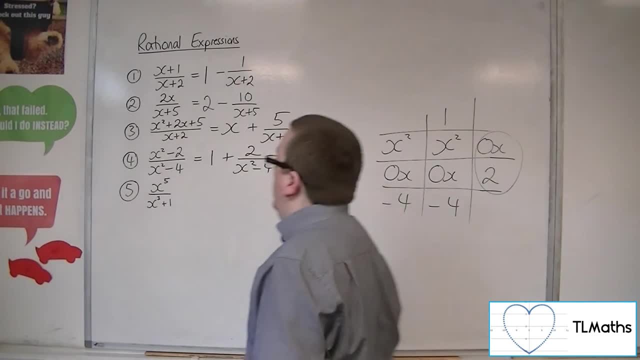 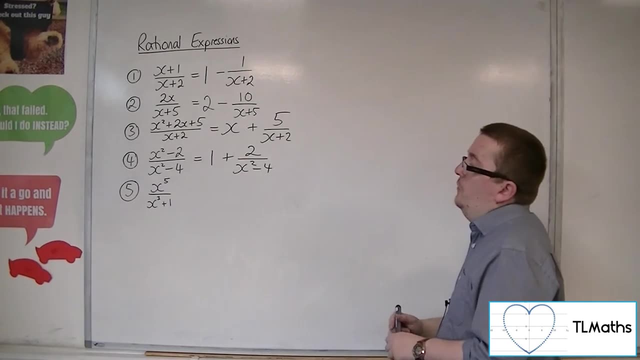 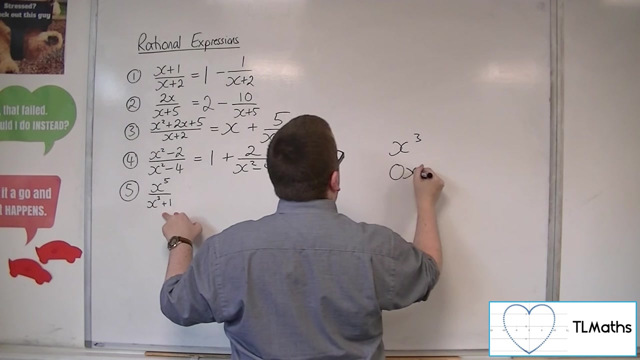 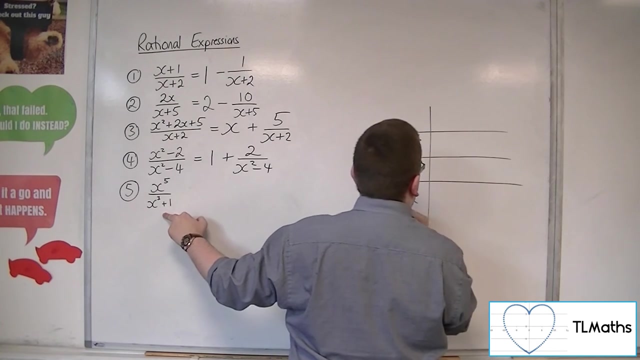 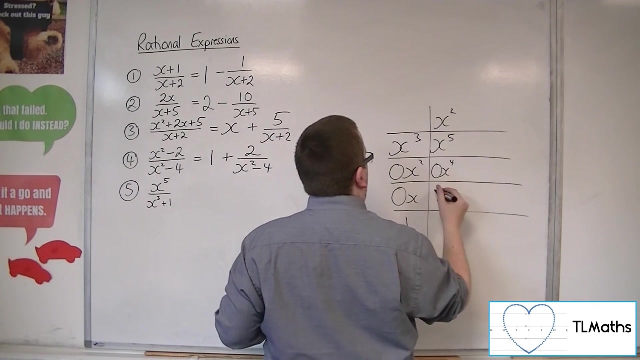 And then finally number 5.. You've got x to the 5 over, x cubed plus 1. So x cubed, 0x squared 0x and 1. So x to the 5.. So x squared, 0x to the 4, 0x cubed and x squared. 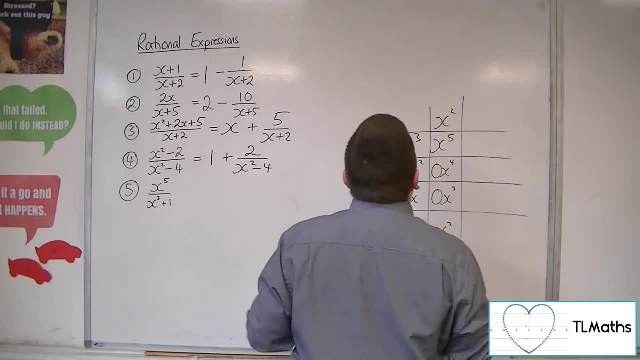 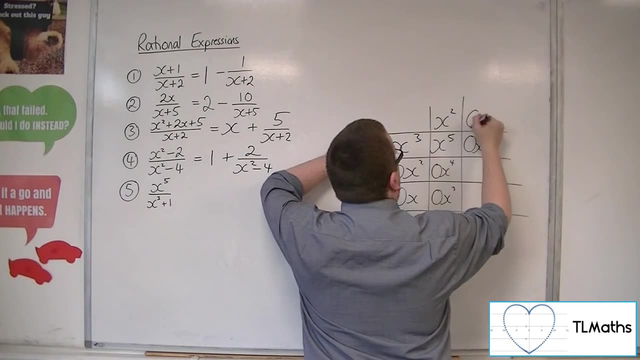 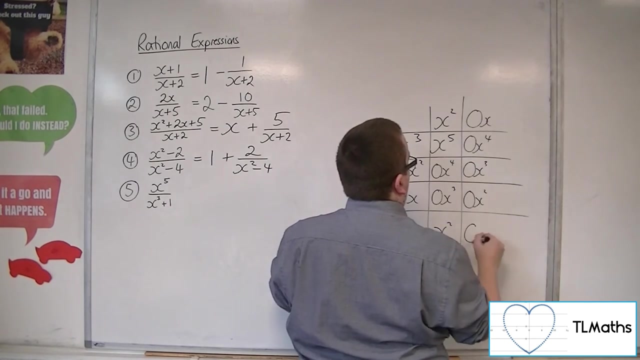 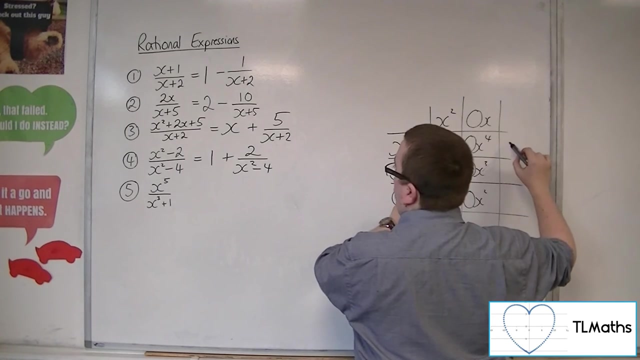 Okay. Well, I don't want any x to the 4's, So I'm going to have 0x there. 0x cubed, 0x squared, 0x, 0x. Okay, Now for cubes. I don't want any cubes. 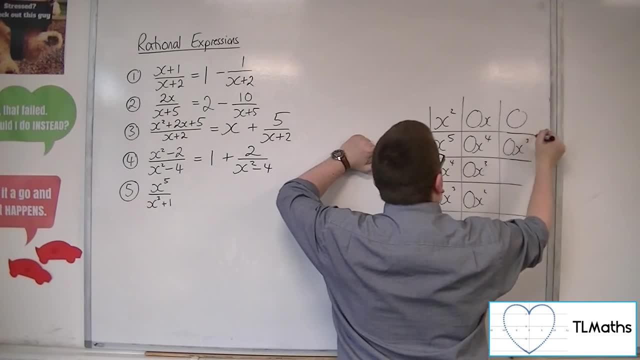 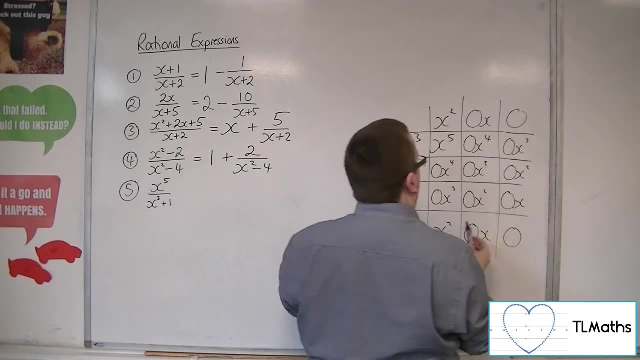 So 0x cubed there, So that'd be 0.. 0x squared, 0x and 0.. Now the 0x squared. well, there's x squared, So I don't want any x squared. 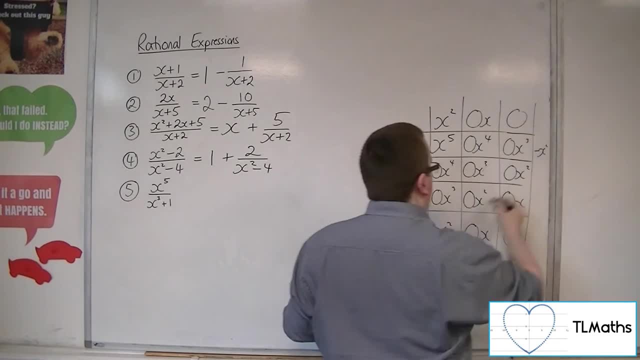 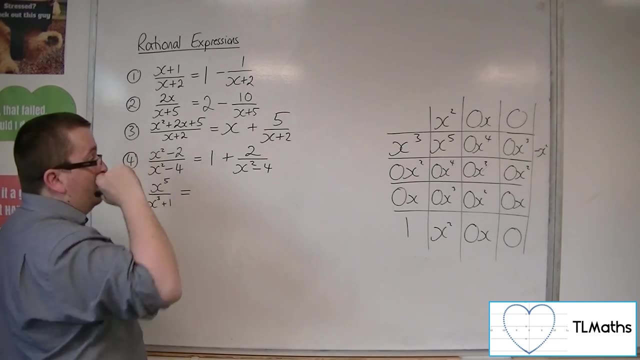 So I'm going to have to have minus x squared up there. So I'm going to cancel that x squared And that's my remainder. So I would have the x squared in the numerator. Oh sorry, the x squared up here. 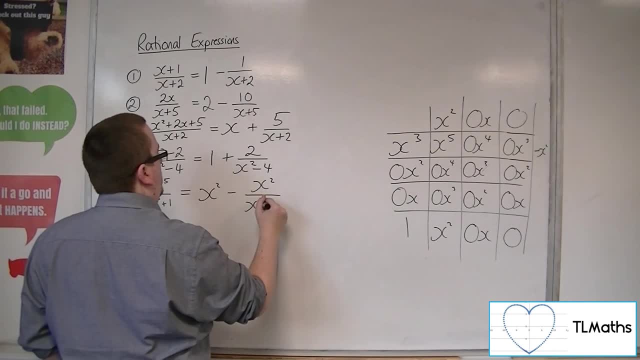 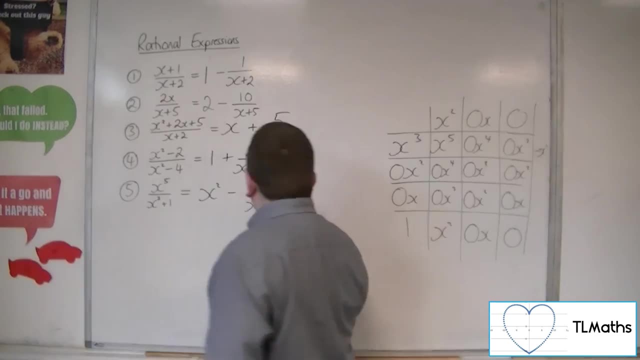 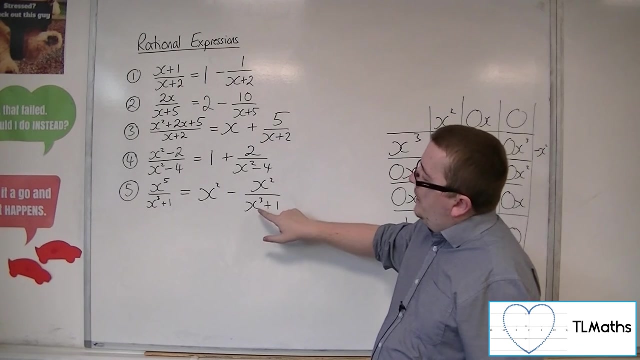 And then I've got minus x squared over x cubed plus 1.. So as x increases, this fraction will be overpowered by the denominator. The x cubed will increase faster than that x squared, And so the denominator overpowers the numerator, so that as x increases, this fraction gets closer and closer and closer to 0.. 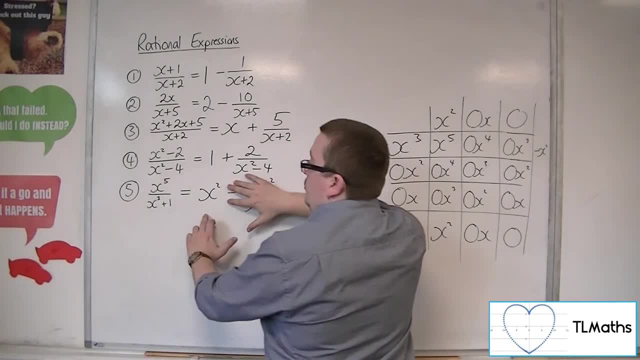 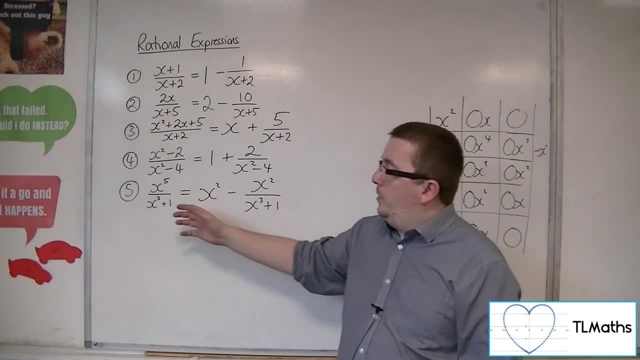 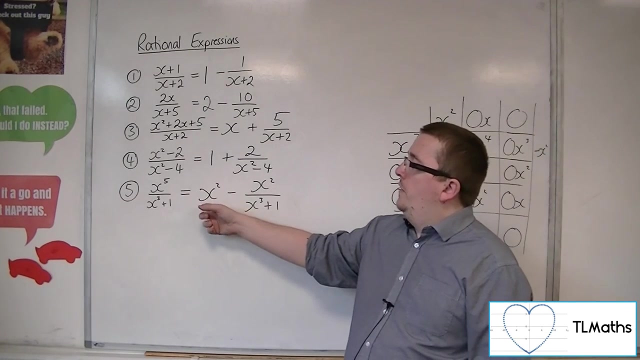 And so this curve will approach the curve y equals x squared as x increases in either direction. So if you plotted y equals x to the 5 over x cubed plus 1 on Desmos or Autograph and you overlaid, y equals x squared. 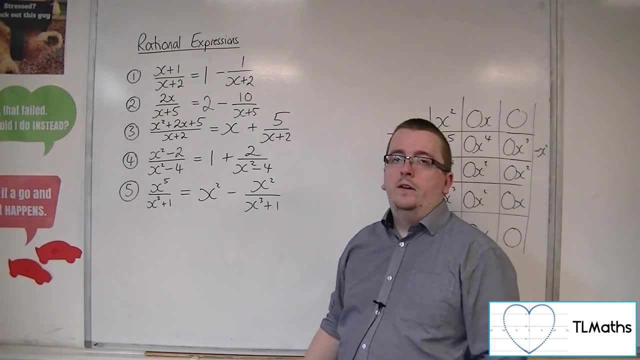 you'll see that that curve will approach that one as you zoom out.